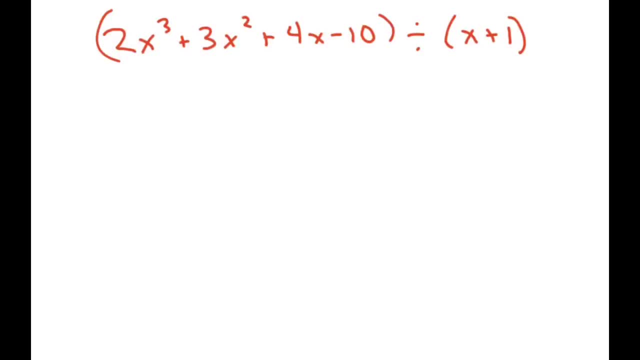 And I know if you've already done this before. you set it up differently, But it's the same process, So the way I set it up is: I know that I'm going to set this to zero. This is my divisor, so that would be: x is negative 1.. 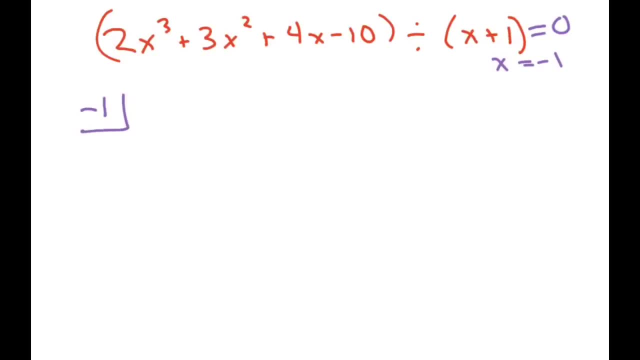 And the negative 1 is what I put in a little box. Then I just write my coefficients. knowing so, I'm going to write 2,, 3,, 4,, negative 10.. And make sure you have this in descending order. 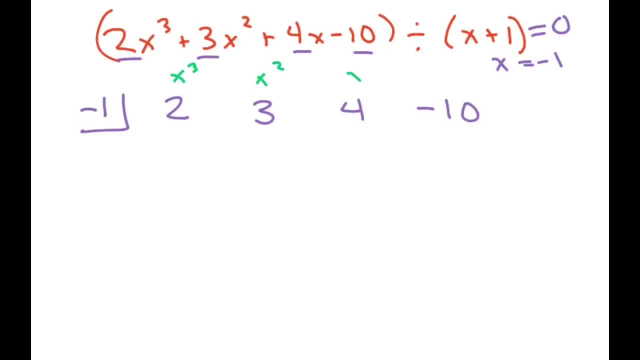 So this would be your x cubed, x squared x 1, and this would be x to the zero. x to the zero equals 1,, by the way. Alright, so then I draw a line here, And the first step you have to remember is to bring down your first number. 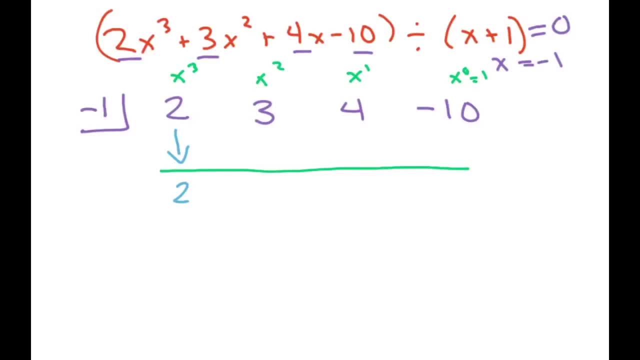 So 2.. Then what's nice about synthetic division is you get to add Versus long division, where you have to subtract So less errors occur. So we're going to multiply: negative 1 times 2 is negative 2. And you put it right there. 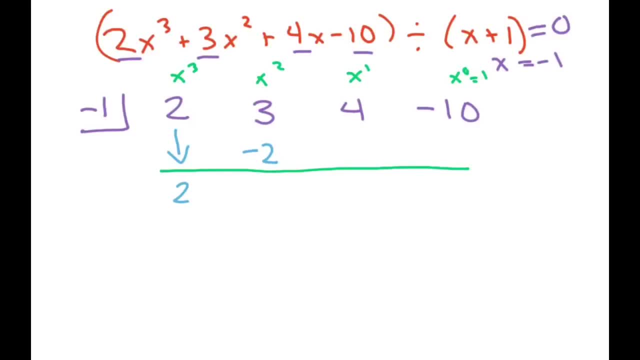 And then you add those or combine those, So 3 plus a negative 2. So it's just basically: 3 minus 2 is 1.. Now multiply these two again, You get negative 1.. Put it there and you combine. 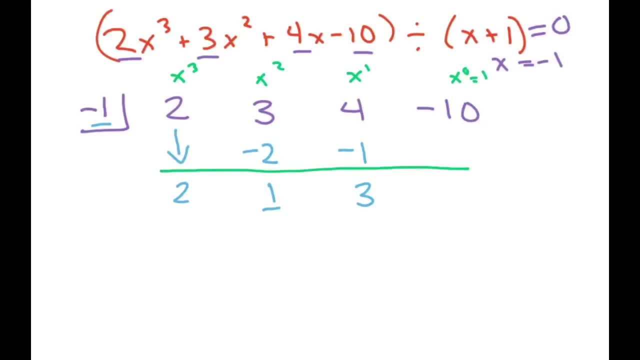 4 minus 1 is 3.. And then you multiply the negative 1 times 3. You get negative 3. And then you combine And that's negative 13.. This last piece- and I always put a box there- is your remainder. 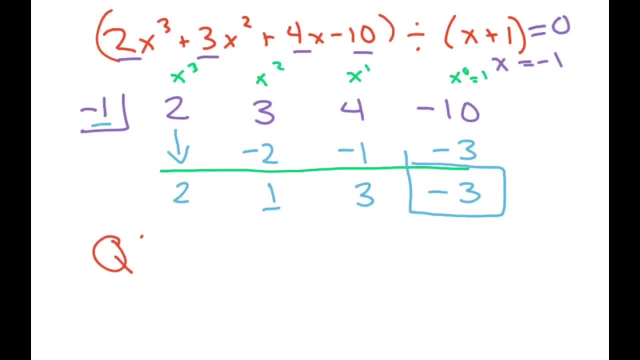 So your quotient And you go down 1. Since we started with 3. You go down 1.. So that's going to be 2x squared plus 1x, which is x plus 3. And your remainder equals negative 3.. 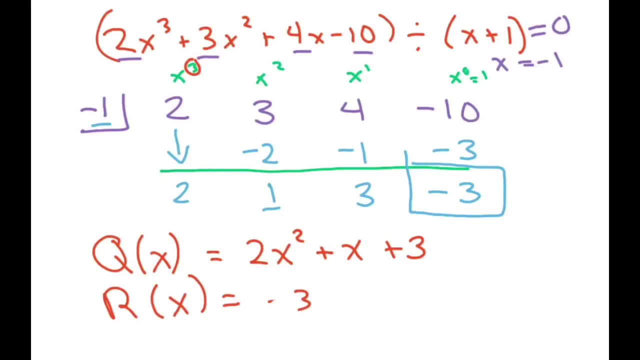 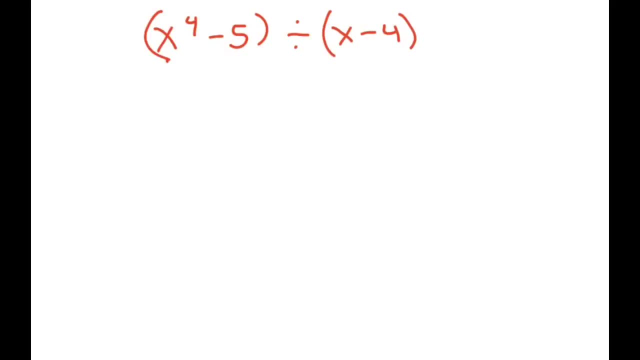 I just want to see how they wrote it. All right, Negative 3.. And the last one is this one. The problem with this one is, well, first of all, if you set this to 0, you get x equals 4.. 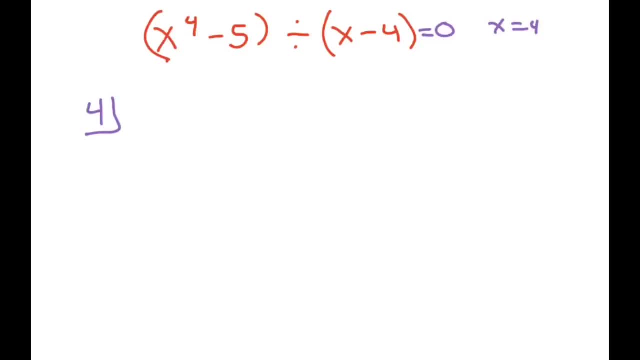 So that's what I'm going to put here, And now what I'm going to have to do. I'm going to have to go x to the 4th, x cubed, x squared, x1, and x to the 0..